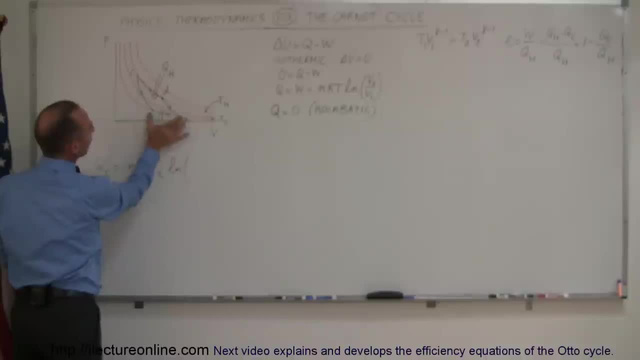 log of v final over v initial. So in this part of the cycle, in this process, v final is vb and v initially is va. so we write vb divided by va. Now to find the heat being put into the system or into the cycle at the hot. 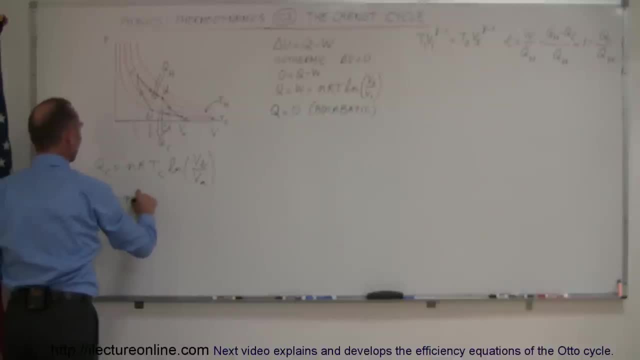 temperature. we have qh and that is equal to nr times temperature, h times the natural log, and again that would be v final over v initial, so it would be vd over vc. Now there's a mathematical trick here. we're going to take the negative of this, but in other words, if I put a negative sign in front, 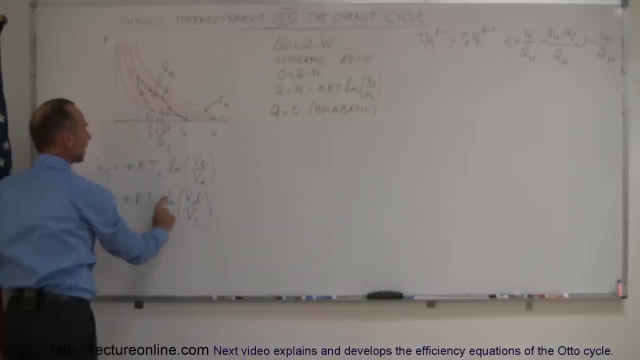 of that and I exchange vc and vd, then that makes that negative as well. they cancel each other out. so I can write: qh is equal to the negative of nrth times the natural log of vc over vd. Remember when you, when you interchange those two variables, that becomes negative and that's not negated by the 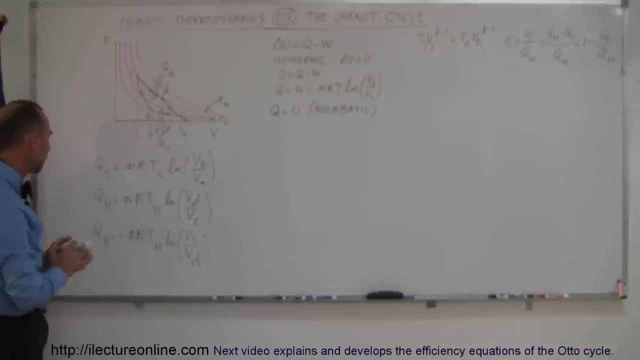 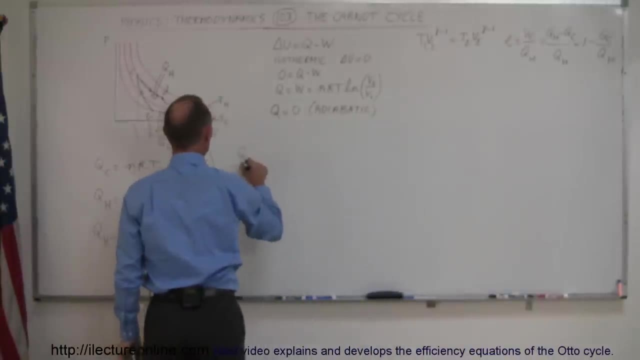 negative over here and again. there's a reason why we did that: because the next step we're going to divide q cold by qh to get that right there. So q cold divided by qh can now be written as this right here, which is nrt: cold times, the natural log of vb over va. 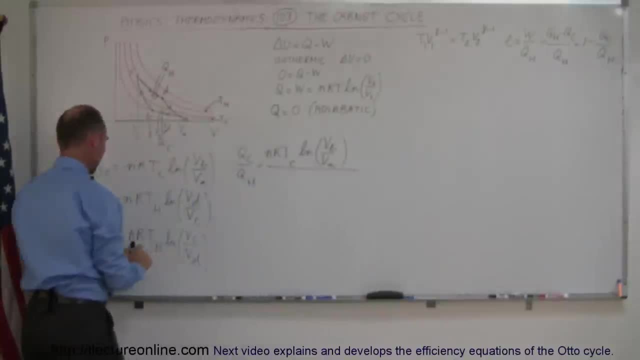 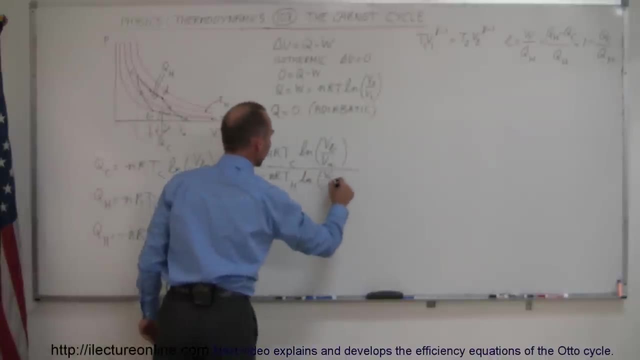 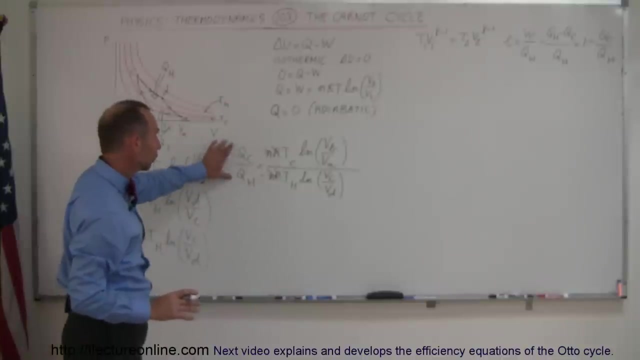 that's this right here, divided by the negative of nrth times, the natural log of vc over vd, and now, right away, you can see that the n and r cancel out, and now we have tc over th and the natural log of vb over va times, the natural log of vc over vd. so that's equal to q cold over q hot, which is 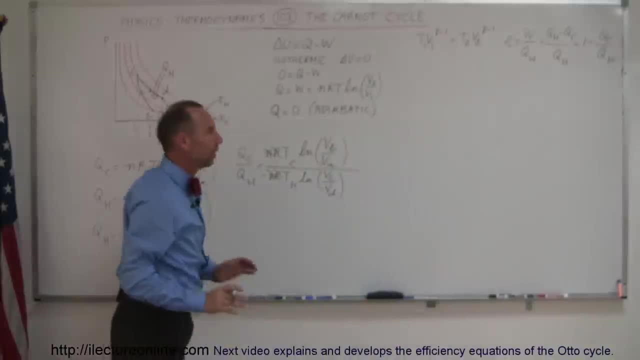 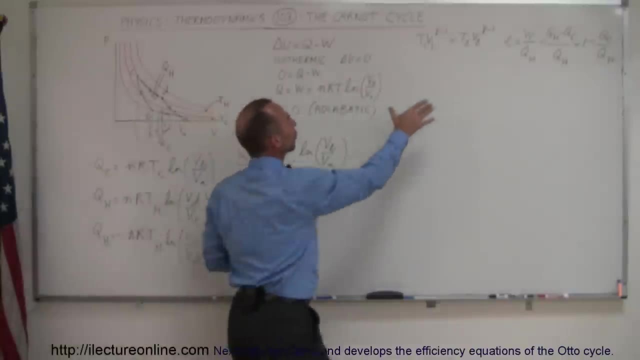 the part of our efficiency equation we have over there. So the next thing we're going to do is look at the adiabatic part of the cycle right here- the two adiabatic processes- and use this equation to relate temperature to volume as well, and then we should be able to solve those two. 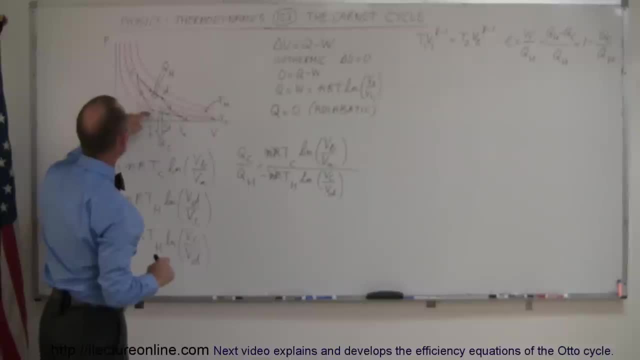 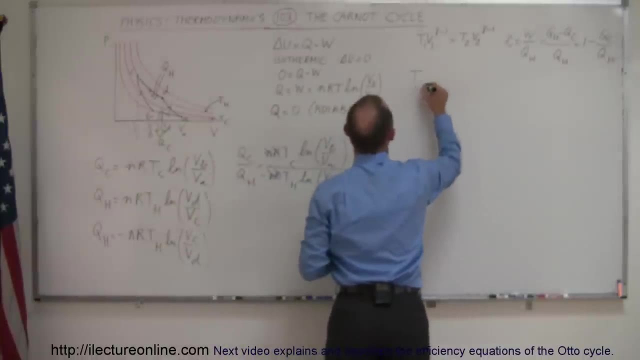 equations simultaneously. So to solve the negative and the negative equations of these two, we should, Starting with going from B to C, we can write temperature at B and, of course, temperature at B is T cold times, V at B and V at B. well, let's simply: V at B to the gamma minus 1 equals temperature at C, which is T hot times V at C to the gamma minus 1.. 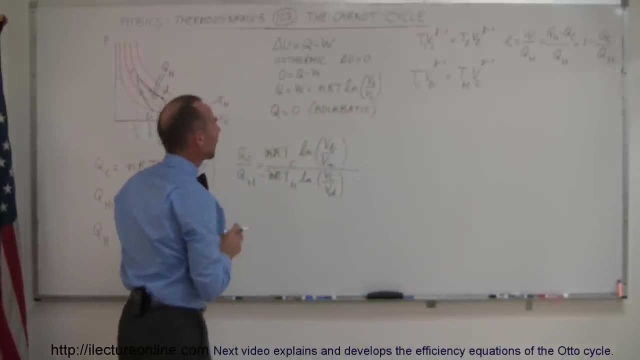 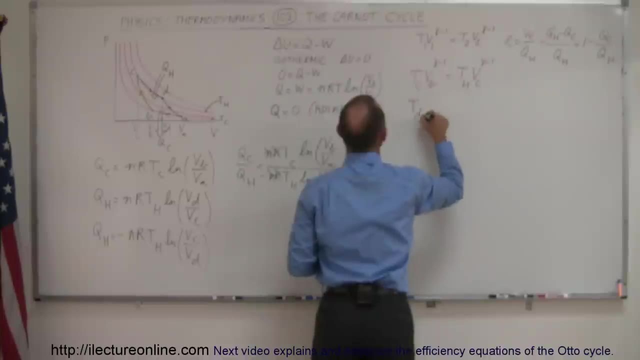 Now we can also do that for the other process right here, going from D back to A, so we can say T at D and of course T at D. that would be T hot. so T hot times V at D to the gamma minus 1 is equal to when we get over here, that would be T cold times V sub A to the gamma minus 1.. 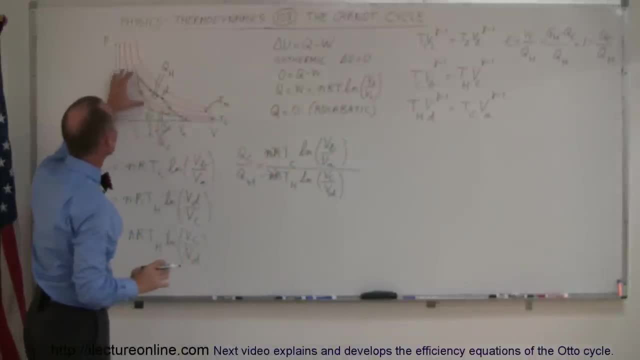 So we use that equation to relate B and C and D and A, because that's an adiabatic process and that's an adiabatic process. Now what I need to do is I need to somehow get rid of the T C and T H here. 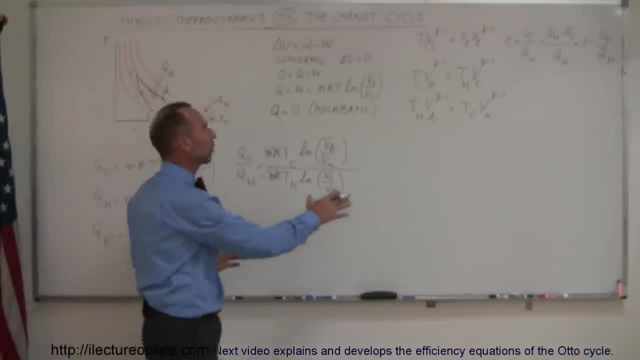 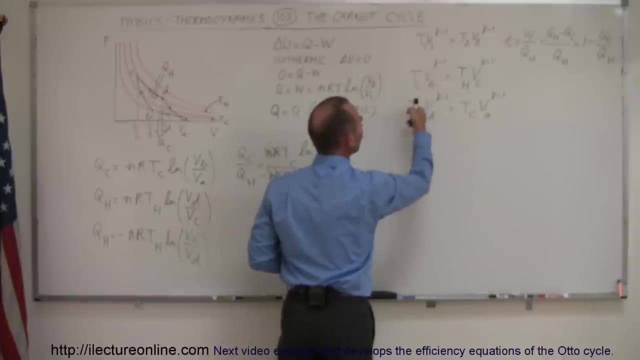 Alright. so how do we do that? How do we get rid of the temperatures in these equations right here? Well, if I divide this equation by this one, but turn around, then I have T C's lined up, I have T H's lined up, and then I think those will dry. 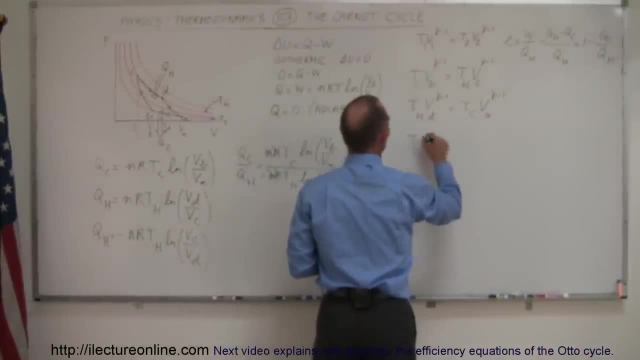 So let's try that. So we're going to take T C V B to the gamma minus 1 and set equal to T H times V C to the gamma minus 1 and we divide that by this equation, but turn around: I get T C V A to the gamma minus 1 and on this side I get T H times V D to the gamma minus 1.. 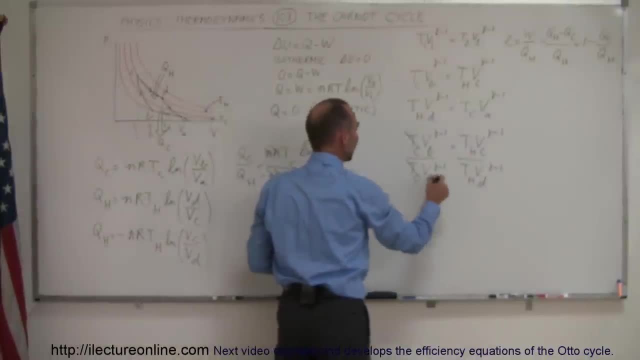 Notice what we've done here. You can see that the T C's cancel out and the T H's cancel out and then you combine the V B to the gamma minus 1.. So we can write that V B over V A and V C over V D. so we can write that V B over V A to the gamma minus 1 equals V C divided by V D to the gamma minus 1.. 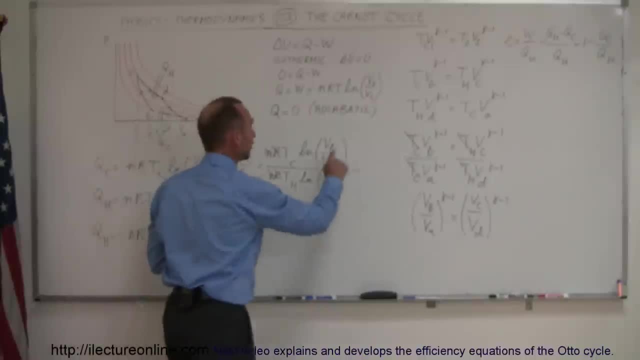 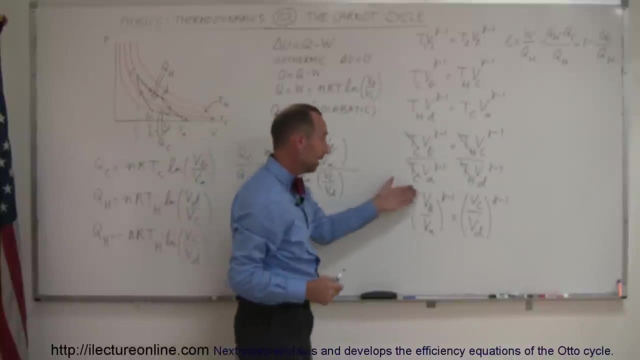 Now, why did I do that? Well, take a look at this equation again. I have V B over V A and I have V C over V D, which is exactly what I have over here. And you can say here then that if V B over V A to the gamma minus 1 equals V C over V D to the gamma minus 1, that these ratios 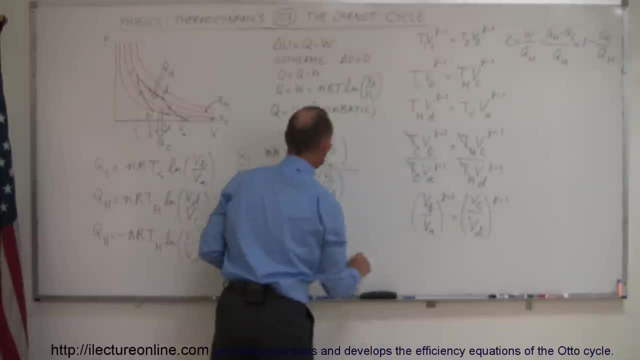 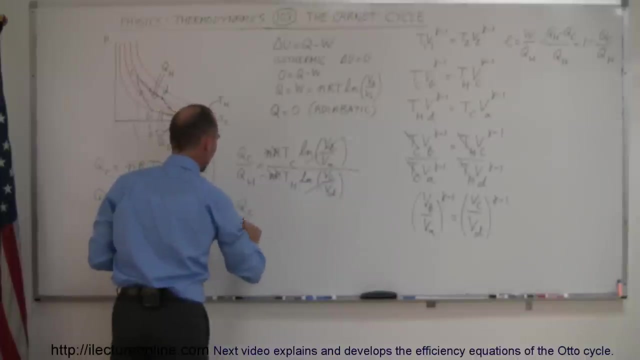 they have to be equal to each other. If those two ratios have to be equal to each other, then this has to be equal to that and those cancel out, because V B over V A is equal to V C over V D, which I have over here. and then I look at this equation and I can write that Q C over Q H is equal to T C over T H. of course, don't forget the minus over there. 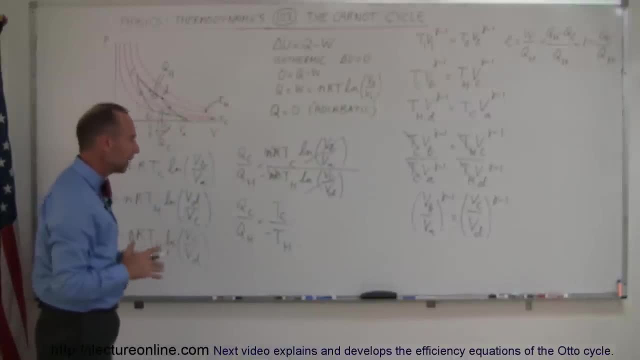 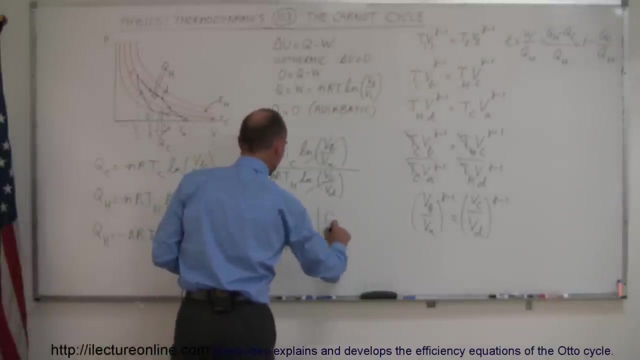 Now, does the minus make sense? Well, it depends. Notice that if I only take the absolute value of the left side, excuse me of that equation, because if I simply look at the quantity, not the sign, and if I then write it like this, if I say the absolute value of Q cold over Q H is equal to, and I can just get rid of this negative sign right here and simply say that is equal to T cold over T H as a positive quantity. 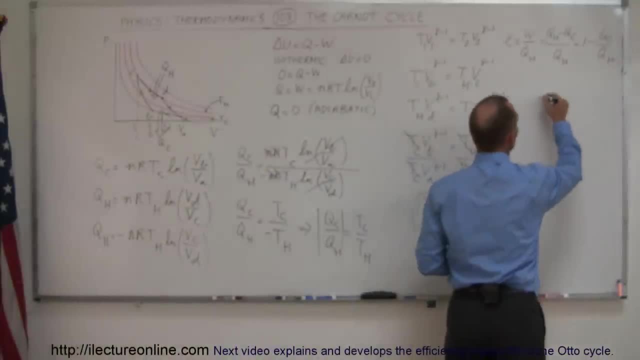 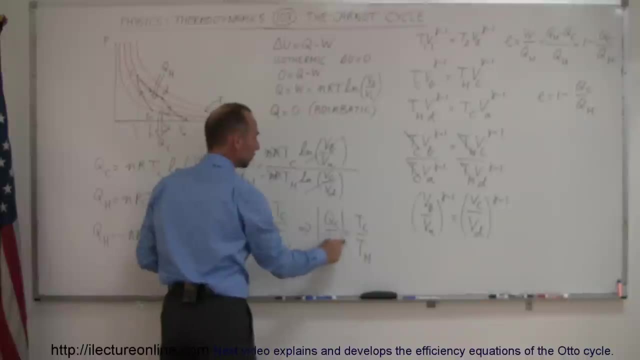 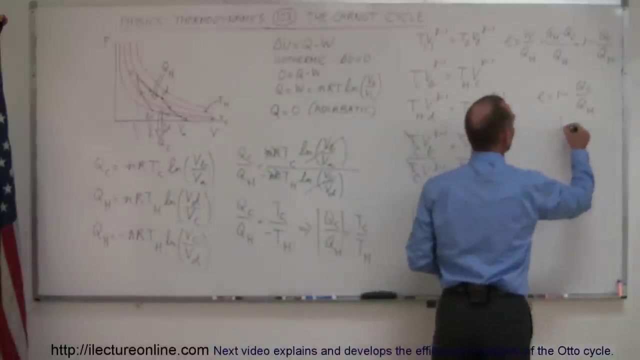 And then I can see over here: if the efficiency is equal to 1 minus Q cold Over Q H, and I have determined that Q cold over Q H is equal to C cold over T H, Then this equation then becomes: the efficiency is equal to 1 minus T cold over T hot for a theoretical Carnot engine. 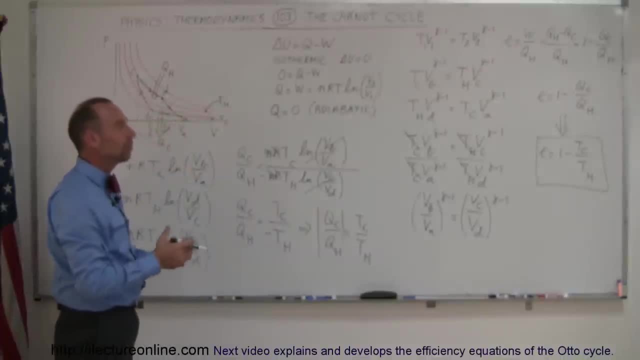 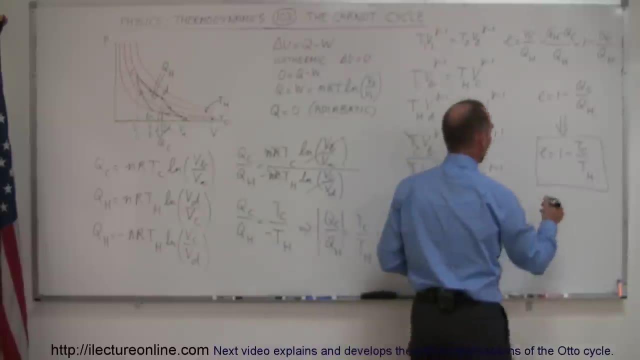 And that then is the maximum efficient. the maximum efficiency any engine can have, simply 1 minus T cold over T hot. Now of course, I can be written in: Okay, Okay, a couple different ways, but also can be written as E is equal to, just like we did there. 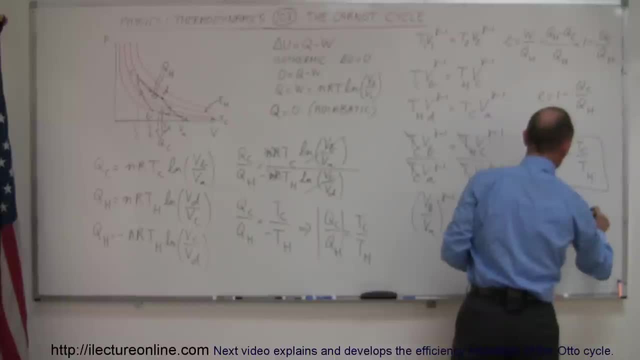 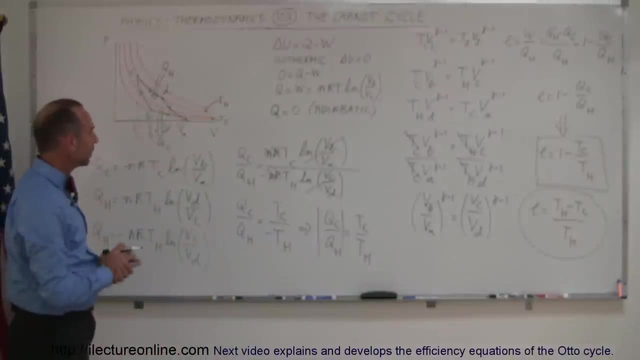 T hot minus T cold divided by T hot, and that's another way of writing the maximum efficiency of a Carnot engine. So that was pretty neat that Carnot came up with this concept that there's no engine with any greater efficiency than this engine right here, Of course not a real engine. 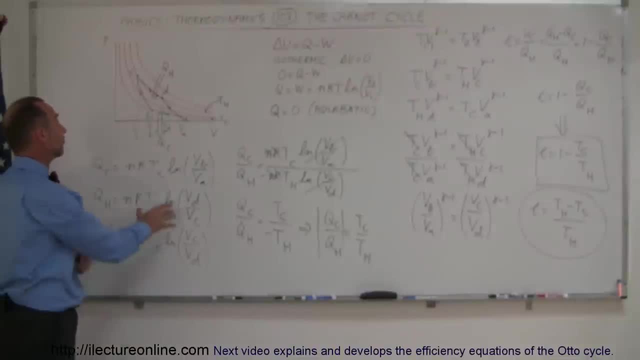 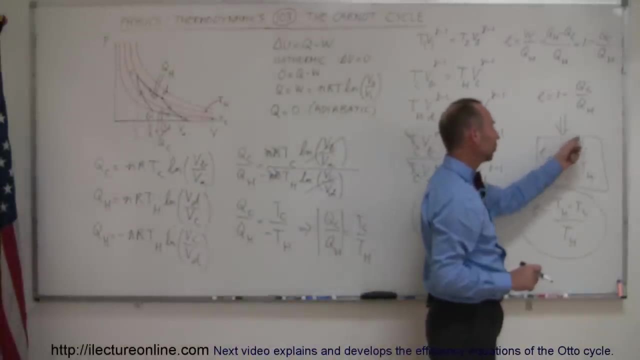 theoretical engine, but at least for engineers, they know that they can never exceed this. and if they want to make an engine more efficient, they can do that by making this relationship as small as possible, meaning make T cold as small as possible and make T hot as.